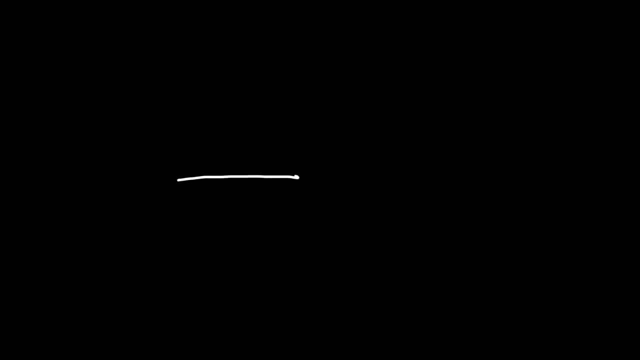 Now in this lesson we're going to focus on calculating the diagonal length of a cube. So let's say the side length of this cube is 9 inches. What's the length of the diagonal? So let's call this a, b, c, d, e, f, g, h. 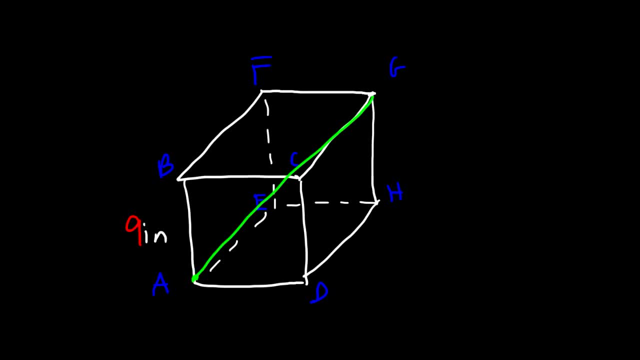 So what's the distance between point a and point g? How can we calculate it? And let's say the side length is x. So let's derive the formula. So first let's calculate the distance between a and h. So if this is x, and this is x, let's call a, h, l. 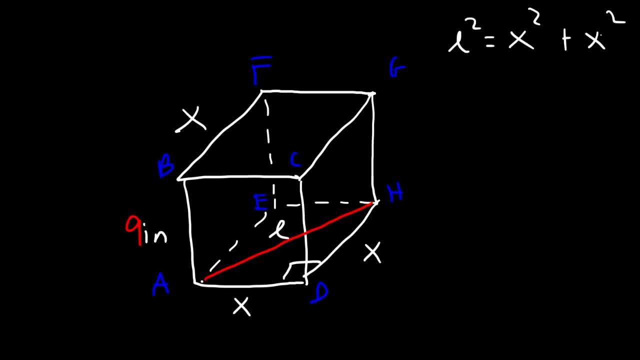 So we can see that l squared is x squared plus x squared, And x squared plus x squared is 2x squared. Now we can draw another right triangle between a, h and g. Let's do that again, And so This side is L, this side is X, and let's call the diagonal length D. 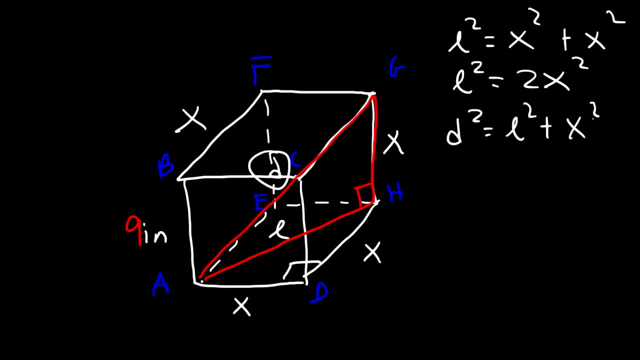 So D squared is equal to L squared plus X squared, And then we could replace L squared with 2X squared, because they equal each other. So D squared is 2X squared plus X squared, or simply 3X squared. So if we take the square root of both sides, the diagonal length for a cube is the square root of 3 times X. 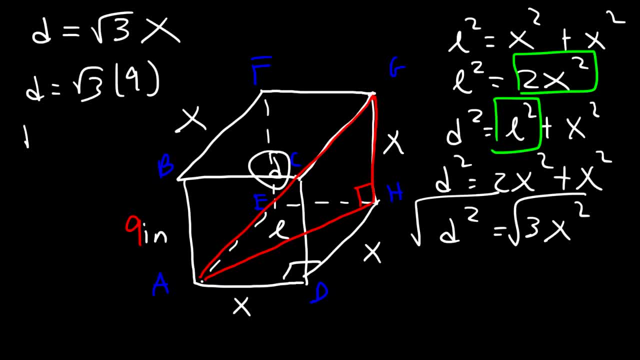 And in this example X is 9.. So the answer is going to be 9 square root 3 inches. So that's the exact answer, And so the decimal value for that is about 15.6 inches. So now you know how to calculate the diagonal length of a cube, if you're given the side length.